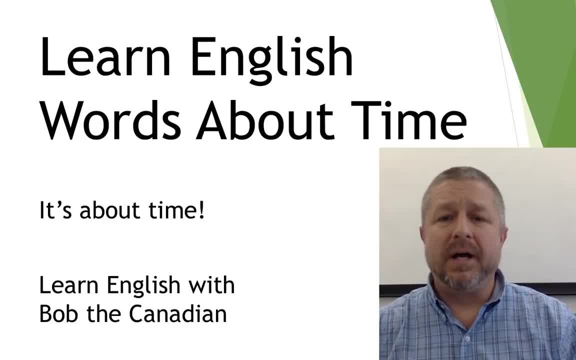 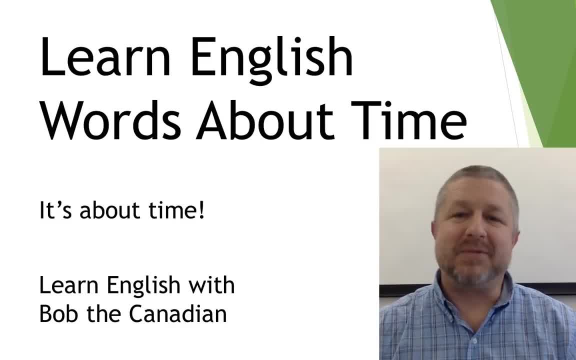 It's something that you express when you say it's about time. It's something that you express when you say it's about time. It's something that you express when you say it's about time, But at the same time, the sentence means that the topic. 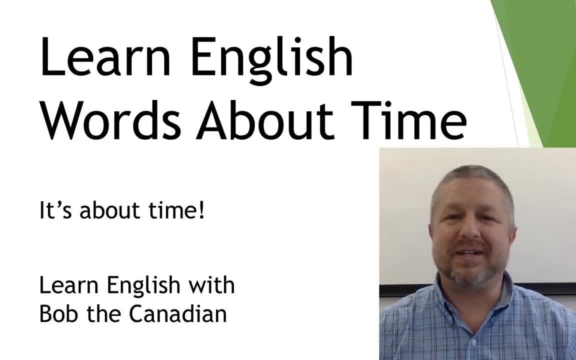 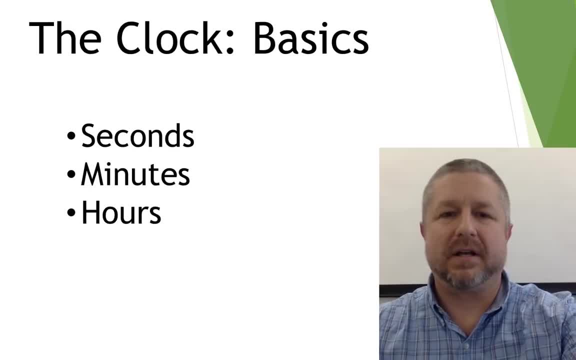 of this video is time. So this is a video about time. Just let me get my slides working here. So I'm going to start with the basics. I'm going to assume that you already know things like seconds, minutes and hours. 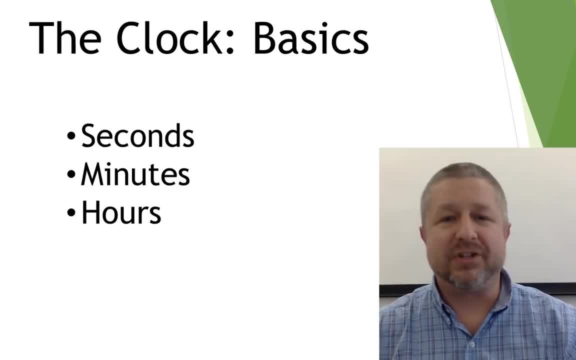 I'm just checking over here. It looks like my stream- health. I'm sure it's fine. So seconds are the shortest amount of time: Very, very little: One second, two seconds, three seconds. Each of those is a second apart, And in most languages second translates as: 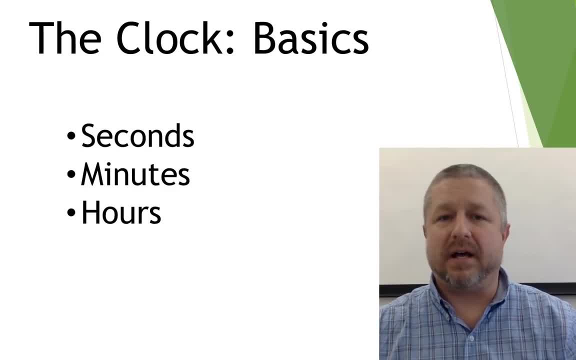 seconds. A minute, then, is the next measure of time: A minute is 60 seconds, And a minute obviously takes a lot longer than a second to go by. And then, lastly, in terms of the clock, we have hours, So hours are 60 minutes make up an hour, So you can also say an hour has 60 minutes. 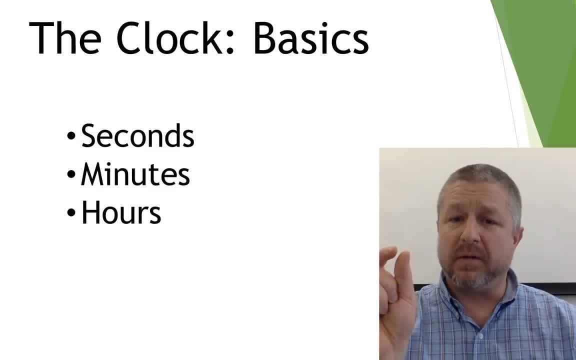 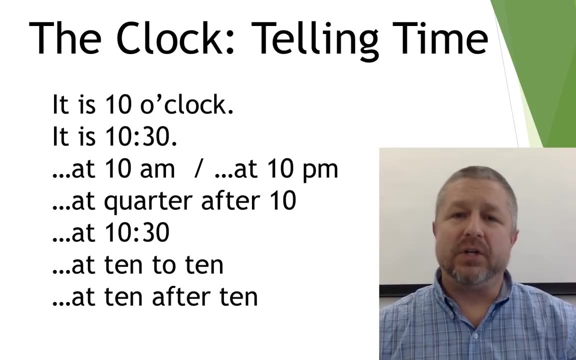 in it. So seconds, very, very small amount of time, Minutes, a bit bigger amount of time, And then an hour is a bigger amount of time next to that. So let's talk about telling time, though, Because this is a little bit different. We're going to use some of the words we just looked. 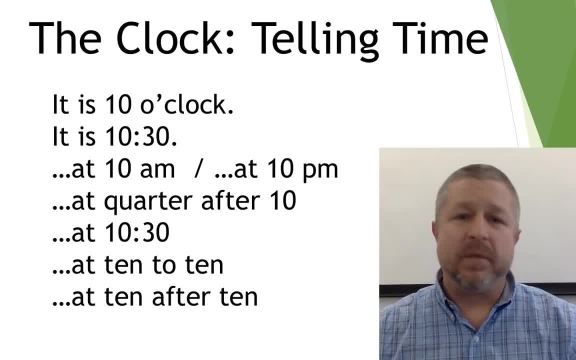 at minutes, seconds, hours to tell the time And, for instance, you can say in English: it is 10 o'clock. You can also say it is 10 or at 10.. What time is it? It's 9 o'clock. 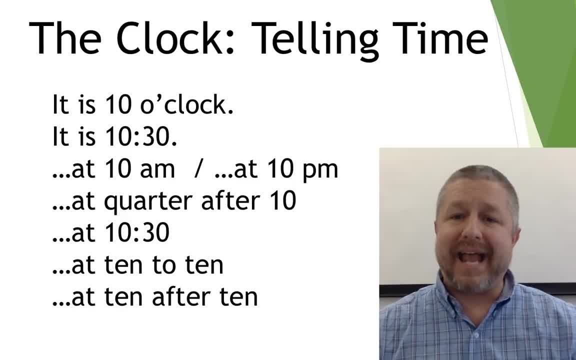 What time is it? It is 10 o'clock In Canada. when we talk about half past the hour, we say it is 1030. We actually say the number 30. I know in other parts of the world they might say it is half. 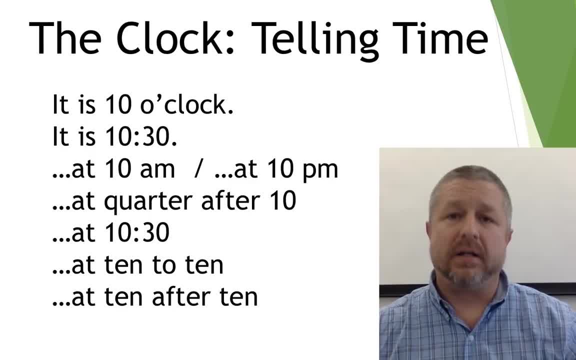 past 10.. You could use that in Canada as well And we would understand what you're saying. But generally in Canada you would say: you would say 1030.. It is 1030.. It is 430.. It is 530,. 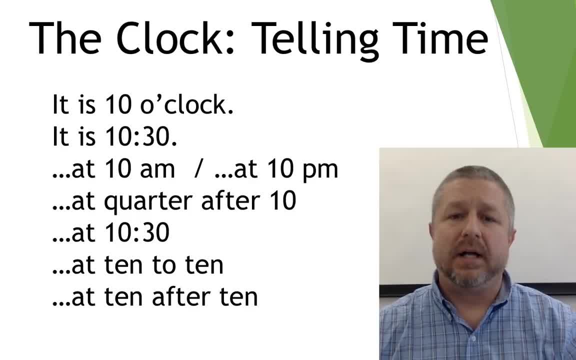 indicating that you are half past the hour. When you reference time in terms of when you reference time in terms of saying, when you're going to do something, you will use the word at. So you could say: tomorrow I have an appointment at 10am. Notice I used: am there We? 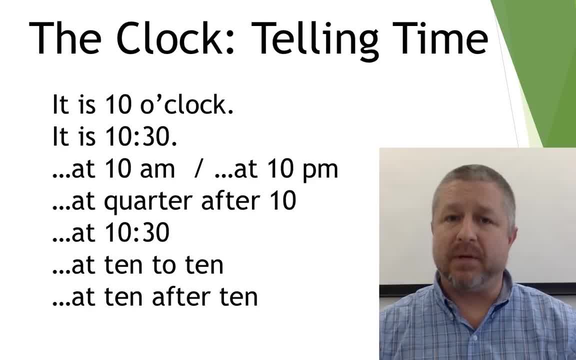 also have am, which means the morning, and pm, which means the evening, But we generally use the word at. So we would say: I have an appointment at 10am, I have a meeting at 10pm, Or I went to. 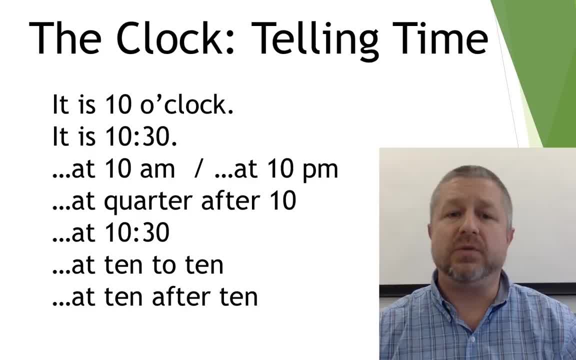 bed last night at 10.. All of those would be valid ways to use time. When you get into, when it's 15 minutes after the hour or before the hour, we actually just say quarter. So we would say at quarter after 10 or at 1015.. You could also say at quarter to 10.. Both of those are equally usable. 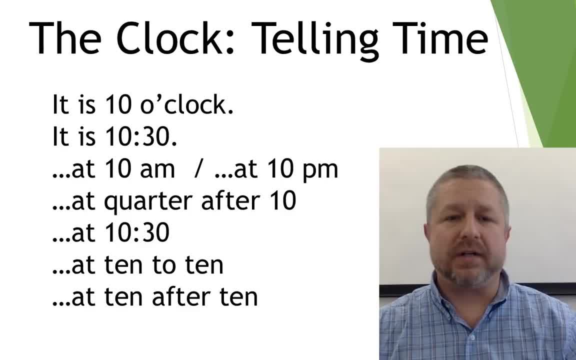 in English And I have in my notes here: at 1030,, at 10 to 10.. So if it was 10 minutes to 10, we say: you know, I'm going to eat my snack at 10 to 10.. Or you could. 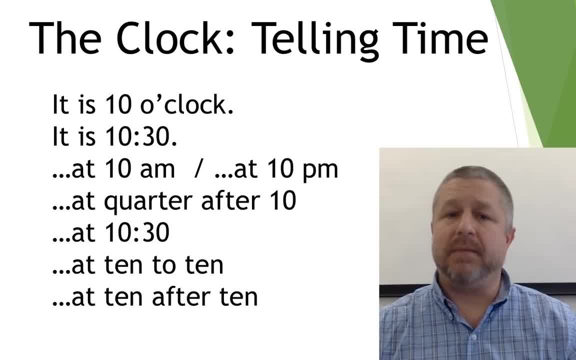 say I'll meet you at 10 after 10, which means 10 minutes after 10 o'clock. Just going to check for questions here. No questions yet, So we'll we'll just keep going. Let me just flip to the next. 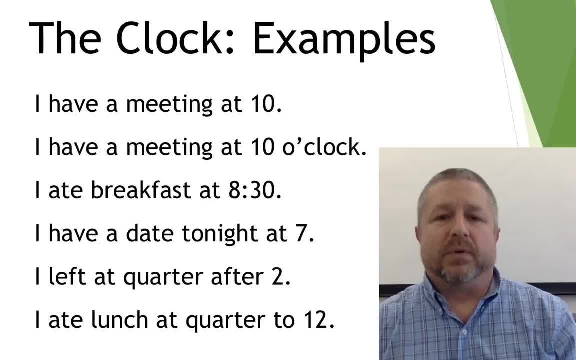 slide. So here I have a few examples And I said some of these examples already in the previous slide. So here I have a few examples And I said some of these examples already in the previous slide. But you could say I have a meeting at 10.. You could equally say I have a meeting at 10. 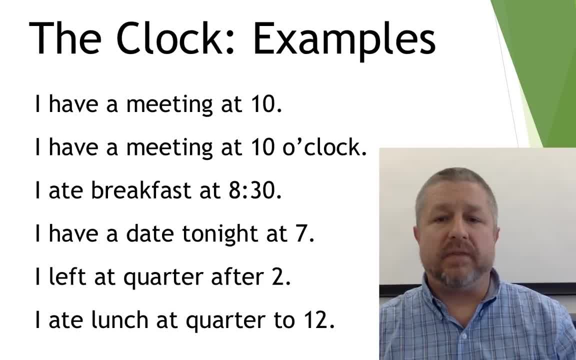 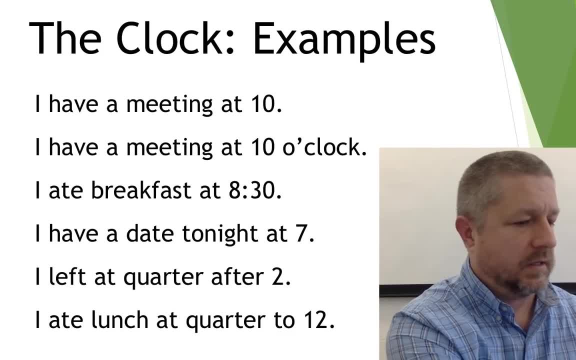 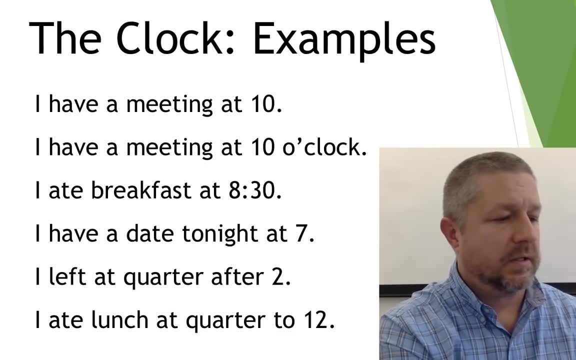 o'clock. Both of those would be would be valid. Let me just check something for a minute. Just want to make sure that we actually have audio on this stream. So now I can't tell if we have audio if I don't talk. So I just want to make sure that we actually. have audio on this stream. So now I can't tell if we have audio if I don't talk. So I just want to make sure that we actually have audio on this stream. So now I can't tell if we have audio if I don't talk. 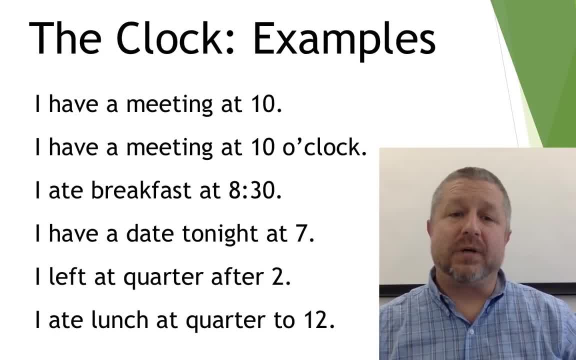 Excellent, So we do have good audio. So again, you could say: I have a meeting at 10.. You could say I have a meeting at 10 o'clock. You could say: I ate breakfast at 830.. And an alternate. 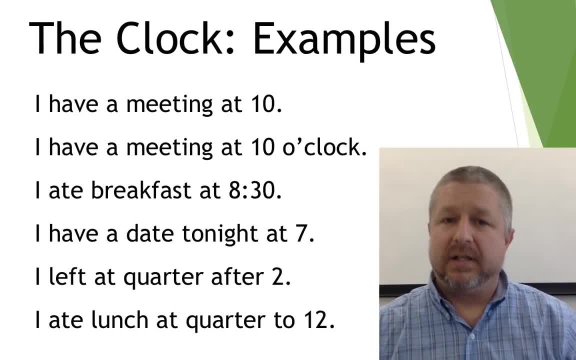 version is to say: I ate breakfast at half past eight. You don't need to say am or pm all the time, You can just say at eight. If you say breakfast, people are going to understand that it was most likely in the morning. You could say: I have a date tonight at seven o'clock. You could say 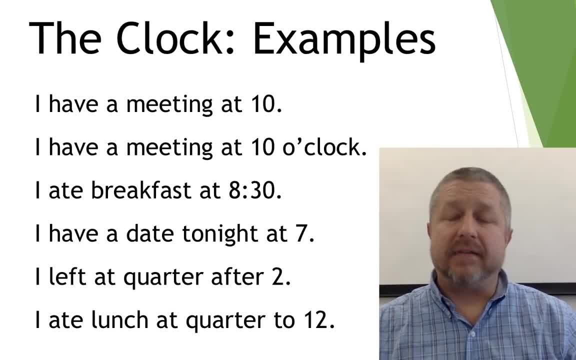 I have a date tonight at seven. I left at quarter after two, So referencing that it was 2.15 when you left somewhere. Or you could say I ate lunch at quarter to 12.. So all of those are examples of using clock time to talk about time. So I have a few people joining in. Hi Rez, Joseph, It's. 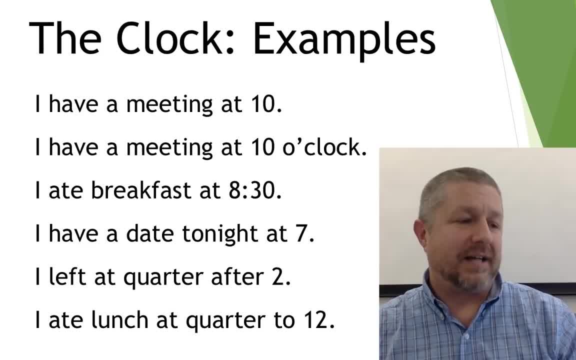 awesome that you're one of my biggest fans, Thank you, And I have Zyvex Saying that I'm awesome, Thank you, Thank you. Thank you very much for that. If you guys have questions in the live chat, please ask them And I'll say them out loud for people who are watching. 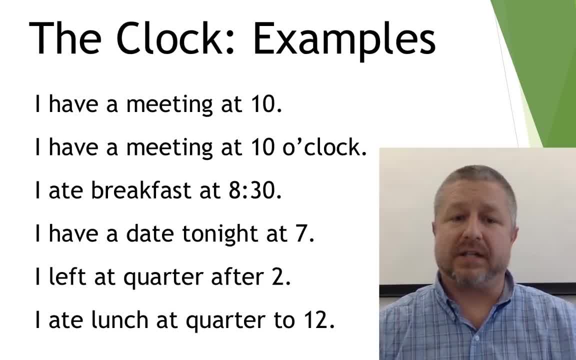 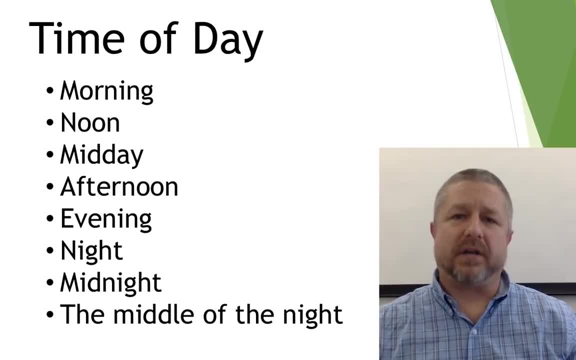 this later as well, But let's move on to the next slide. So time of day. So we have a lot of words to talk about the time of day where we're not actually saying 10 o'clock or seven o'clock, where we reference in general. 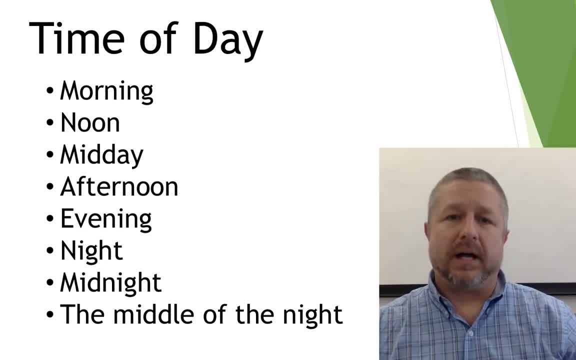 time of day, And some of those are things like morning. I got up in the morning, which is early in the day, Or you could say I had lunch at noon, which is the middle of the day. We don't use the. 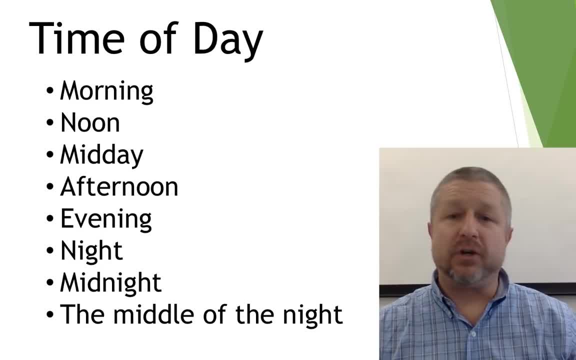 term midday as much, but the term midday refers to the middle of the day And it's probably anywhere from 11 am till 1 pm. somewhere in there You could say midday. After lunch we have what we call. 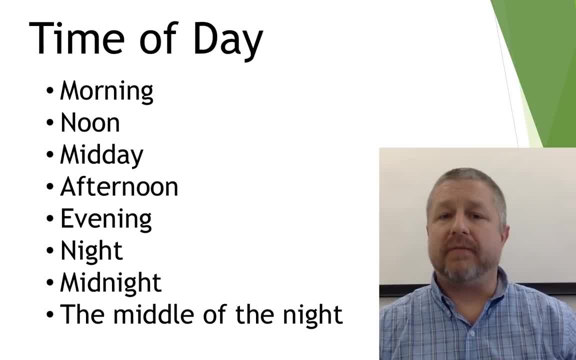 afternoon, So the afternoon, And we have evening, which is towards the end of the day, Usually somewhere around when it's starting to get dark- we would use the word evening- And then, obviously, we have night, which is when it's dark outside. We have midnight, which is 12 o'clock midnight. 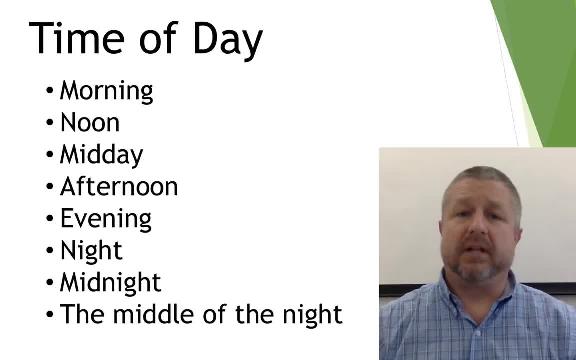 And then we have a little phrase we use sometimes like the middle of the night. So you could say middle of the night because I needed to go to the washroom, Or I was up in the middle of the night because I wasn't feeling well. Let's move to the next slide. If there's any questions, do ask them. 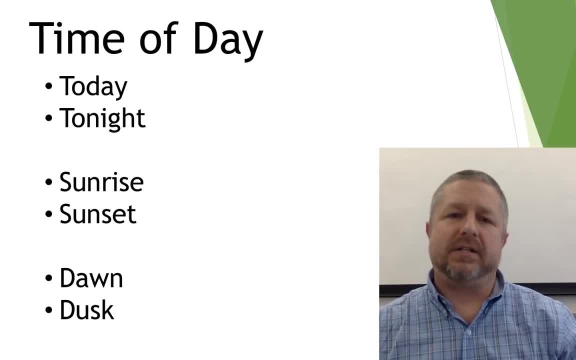 We have a few other general time of day sayings. Obviously, you know today and tonight. Those are very familiar words. I worked today, I will not be working tonight- And they're just used to refer to or the evening time. We also have sunrise, which is when the sun comes up in the morning, So I was up. 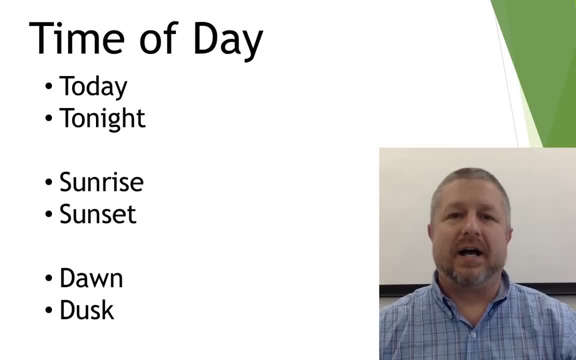 at sunrise. And another little phrase you can use is: I was up at the crack of dawn. That's the earliest time you can get up when the sun is rising. And then we also have the term sunset, which is just as the sun goes below the horizon. we have the sunset And we also have two other terms We have 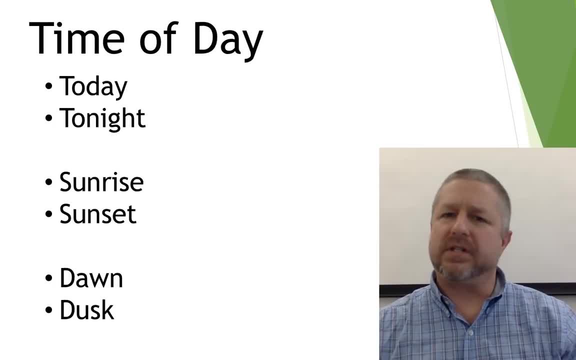 early morning, which is early morning just after the sun has risen, or as the sun has risen. We would call that the dawn, And then the end of the day we have dusk, And dusk is just when it's beginning to get dark. We would refer to that as dusk. So I'm going to stop just and take a question here. 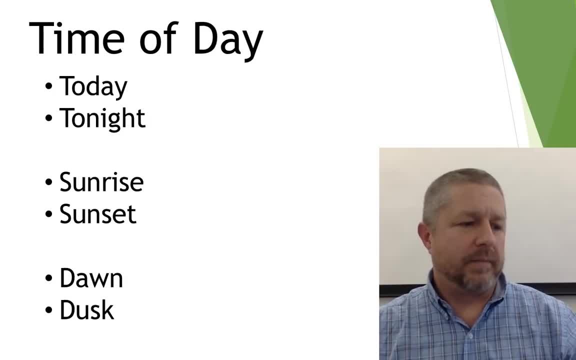 from Rez. He has the question: I heard somewhere that learning English through movies is not very easy. What do you make of that? Well, I actually think watching movies is a great way to learn English, especially if you are watching a movie where you've already read the book or novel that 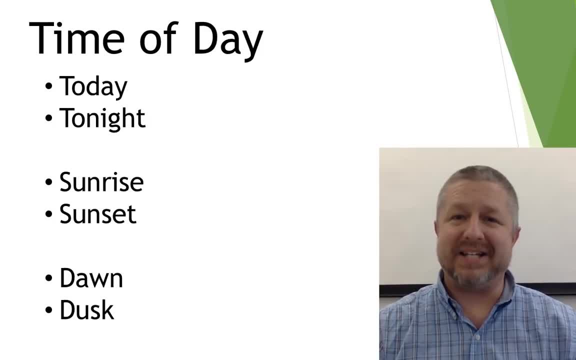 the movie is about, And I know sometimes that can give away the ending, but it is just a good reinforcement. I often recommend that people read a book called The Martian by Andy Weir And then, once you've read the book, to go and watch the movie. 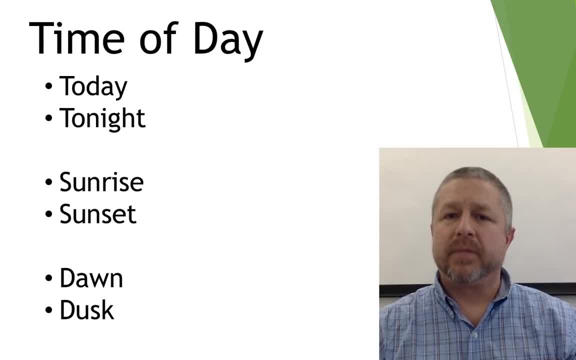 Obviously, watching movies does not get you speaking And obviously watching movies is not the same as writing, But it is definitely a good exercise to read the book and then go to the movie and listen to the movie. So I hope that answers your question. We're going to move on. Next slide here We're. 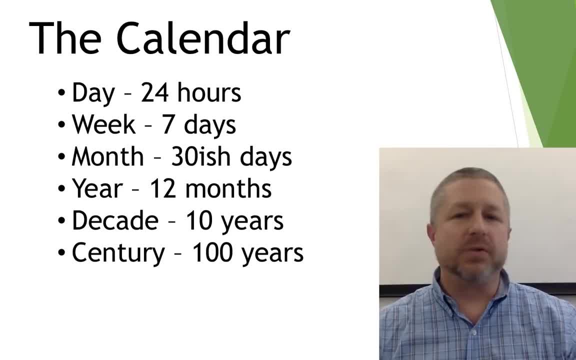 going to talk about the calendar, So I think most of you are aware of this. The point of this video is to help you learn how to use these. So we have day, And a day is made up of 24 hours. We have the week, which is made up of 7 days. We have the month, which, if you notice there, 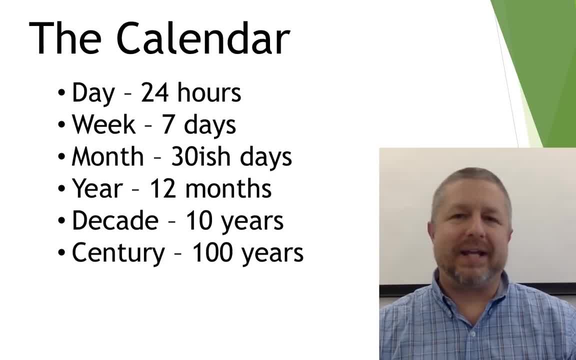 I put 30-ish days. Ish is a way in English to say approximately. So we do know that months can have 31 days and that months can have 28 days in them, But a month is about 30 days or 30-ish days. We 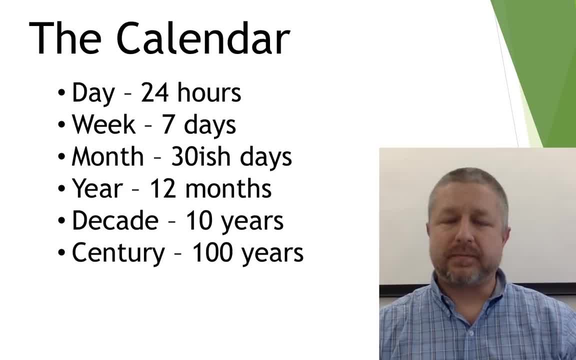 also have the year, which is 12 months. We have a decade which is 10 years And we have a century which is 100 years. And we have a century which is 100 years And we have a century which is 100. 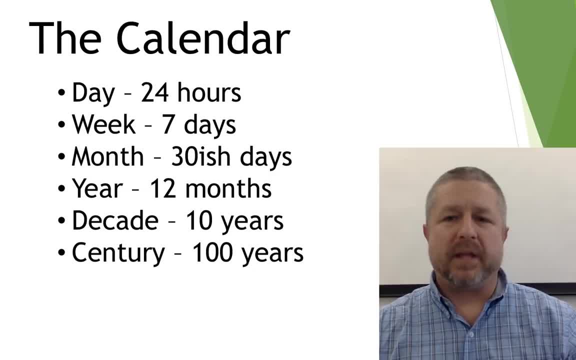 years. So that was a little bit of review. A little bit of review in the sense of you can kind of see how these relate to each other, But let's look at how to use some of these. Oh, I have a few more to. 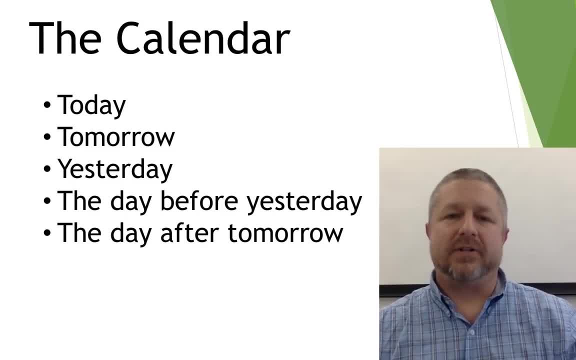 go over first. We looked at today as well in terms of a calendar, But we also have today, tomorrow, which is the next day, And we have yesterday, which is the day before today, And in English we don't really good terms for the day before yesterday. We actually say the day before yesterday, So the day. 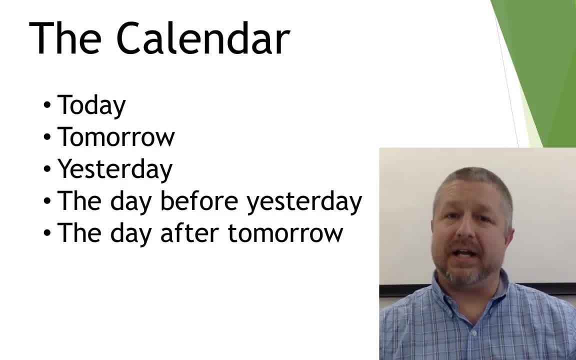 before yesterday. I went shopping Yesterday. I ate some food. The day before yesterday I bought the food And we don't have a good way to refer to the day after tomorrow, So we actually call it the day after tomorrow. So the day after tomorrow I will be going to Toronto to see a show. 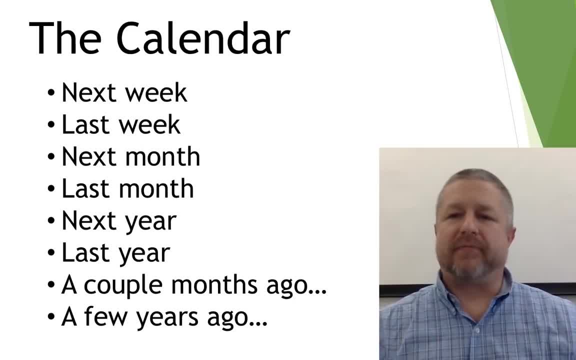 In terms of how you reference forwards and backwards in time. we say things like next week. So if it's not happening this week, you would say that it's happening next week. So next week I'll be going on a trip, Last week I ate a hamburger. So that's in the past. So when you're talking in the future, you 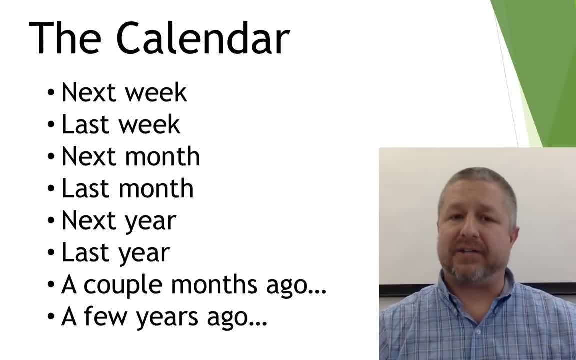 would use next week. When you talk in the past, you would use last week, The same for next month, The same for last month. So last month I went to the dentist, Next month I'm going to see the doctor, And same with next year and last year. You don't use next and last with days. I often hear 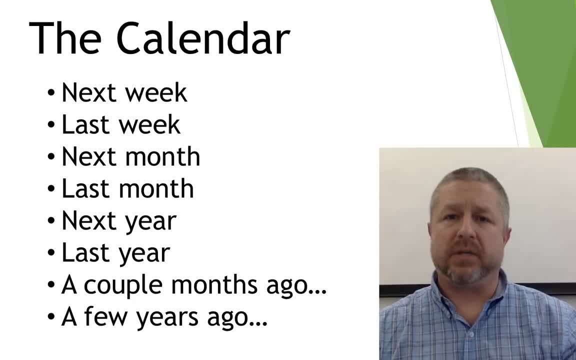 this mistake made by newer English speakers, where they say next day I'm going to school. That is not correct. Don't say next day, You would always say tomorrow. And I've heard new speakers say day Last day, I ate a hamburger. Don't use that either. You would say yesterday And then just a. 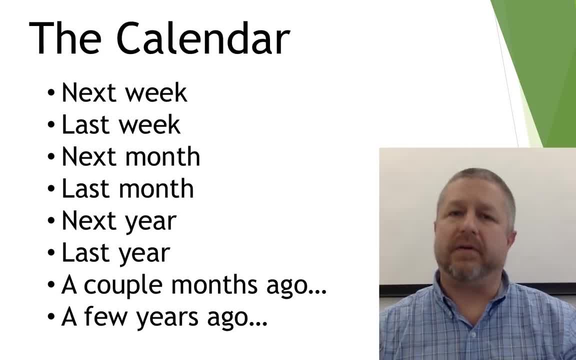 couple of phrases at the bottom, When it's a vague amount of time. you say you know, a couple of months ago I had a holiday. A few years ago I met a friend. So it's when you don't know the exact. 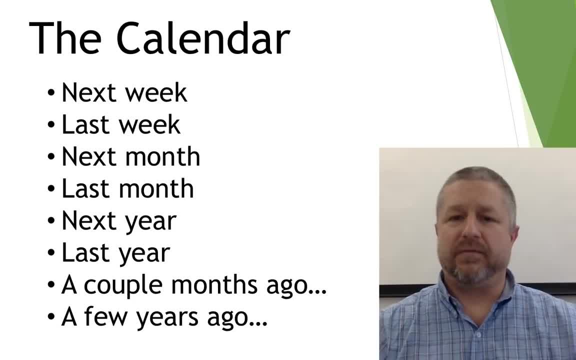 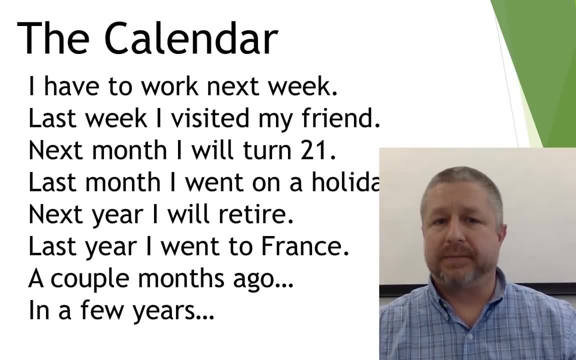 amount of time where you can reference in the future. So here's a few examples with the calendar. I have to work next week, So that's something that's happening in the future. Last week I visited my friend, So that's something that happened in the past. Next month I will turn 21.. Maybe next. 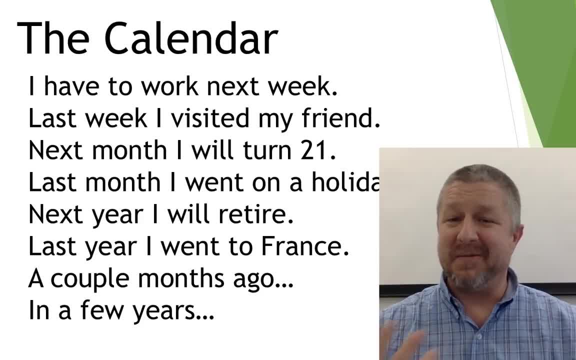 month it will be my birthday. Next month I will turn 21.. I'm a little past 21.. I'm not turning 21 at next month. I'm going to kind of. I'm covered up a bit there, But last month I went on a. 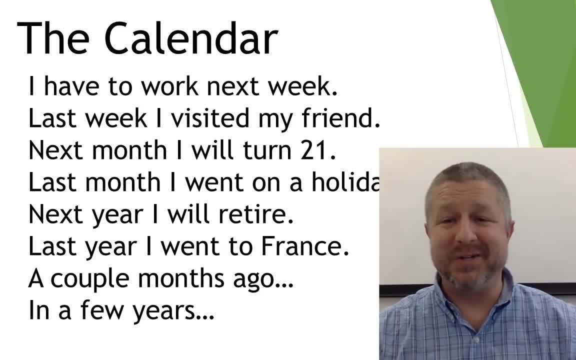 holiday. Next year I will retire. I'm not that old either. I'm not going to retire next year. Last year I went to France, or a couple of months ago, or in a few years. So those are the examples there. 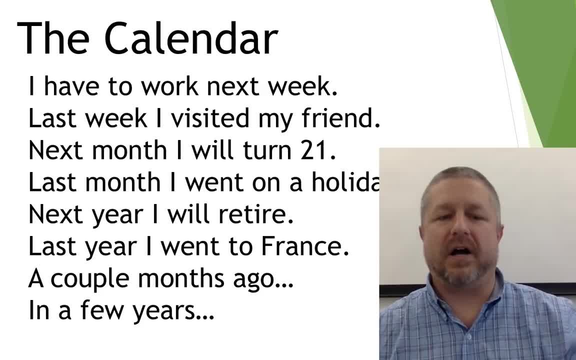 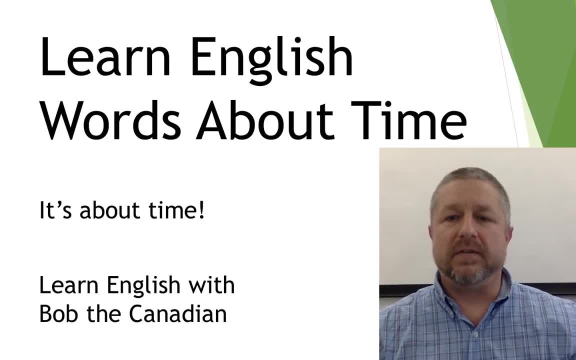 of how to use and reference back and forth in time when you're there. Let me just check. I think the next slide is the ending slide. Yes, it is. So I'm just going to leave that slide up And then, if there are any questions, I'm going to look over at the chat. I will just take some time to answer. 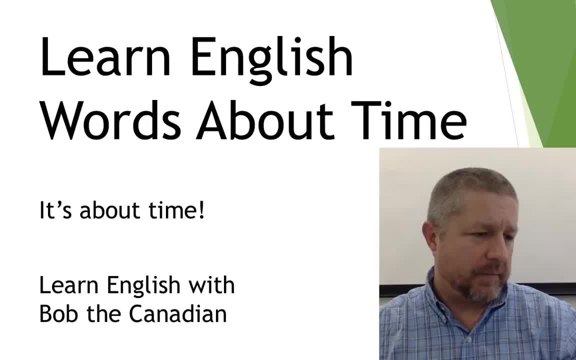 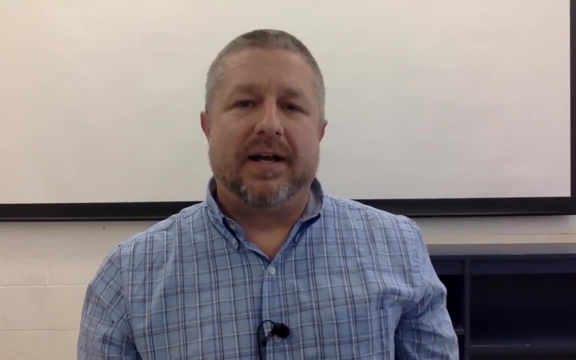 them before we wrap up this live stream. So let me have a look. I'm one of your biggest fans. Which films do you prefer from Zyvex, underscore, Venom? What films do I prefer? I really enjoy films. science fiction films. I enjoy films. I read science fiction books. I enjoy films about 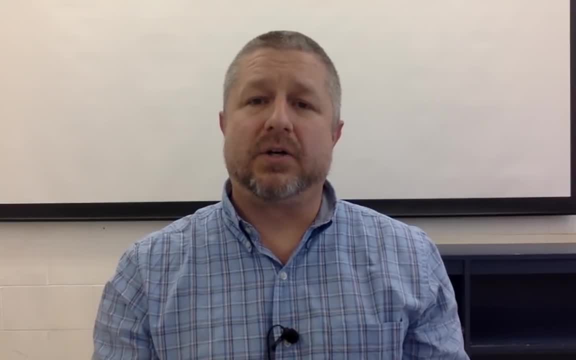 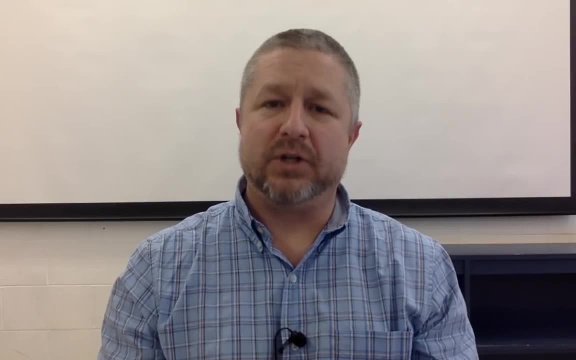 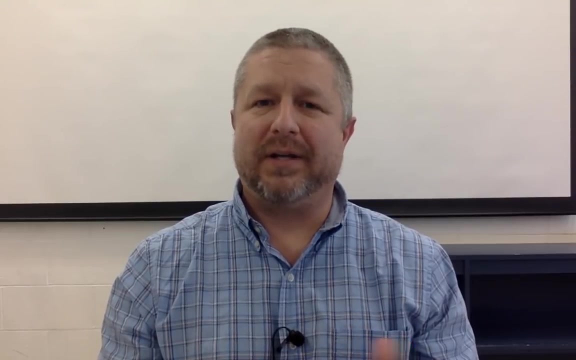 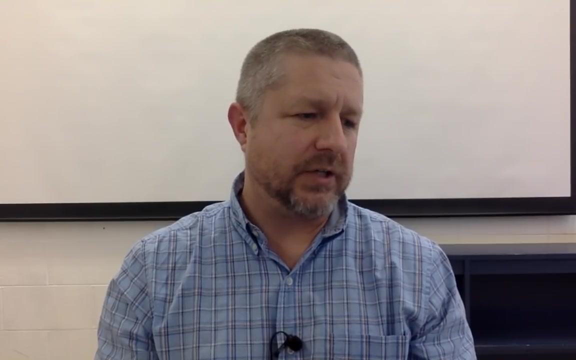 science fiction. I also really really like crime drama, So any film about police detectives, those kinds of things, I really really enjoy those. What do I prefer, though? As long as the story in the film is well written, I will enjoy the film a lot. Do you think traveling abroad to an English-speaking country is? 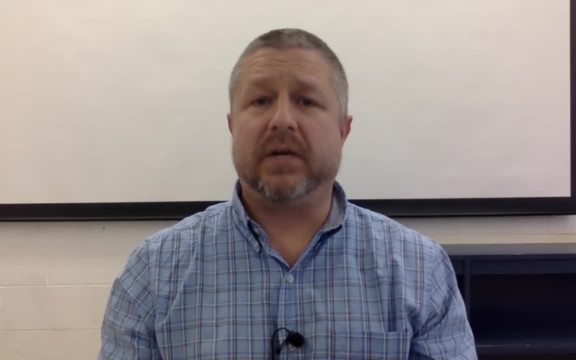 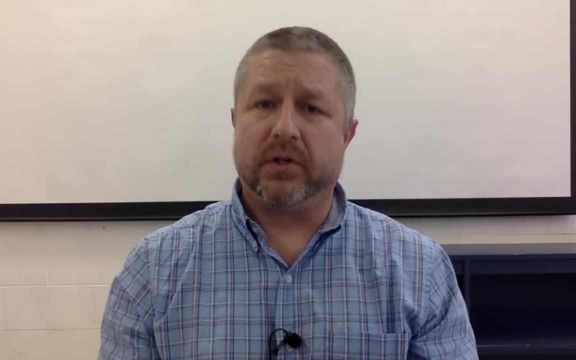 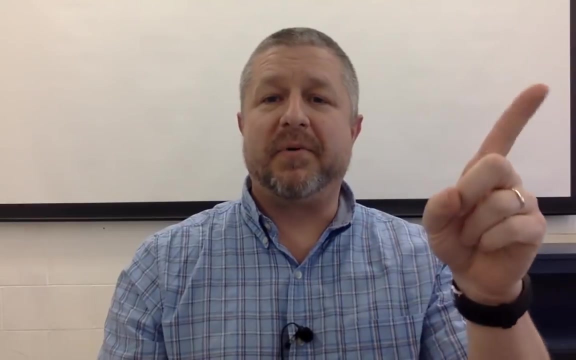 a must-have. So that's another question from Rez. That's a great question, You know. here's what I think: The internet is an amazing tool for learning a language. I'm going to make another video later this week And you can follow the link. I'll put the link up there. Now I know where I'm pointing. I'll put the link. 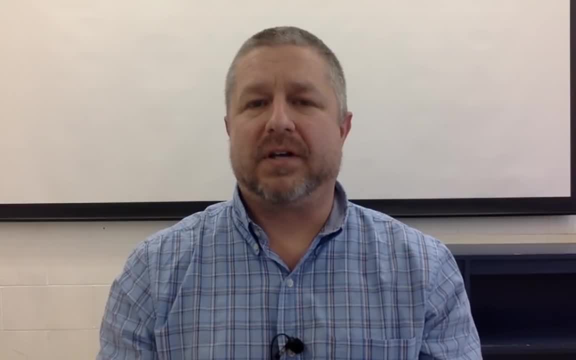 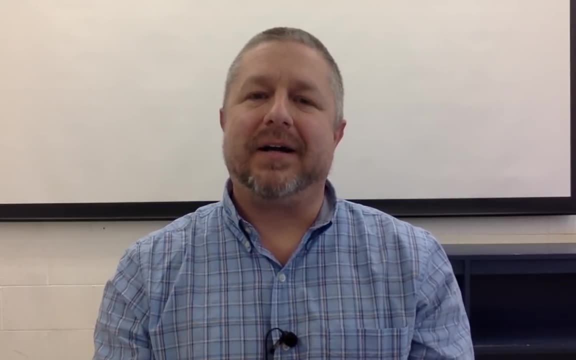 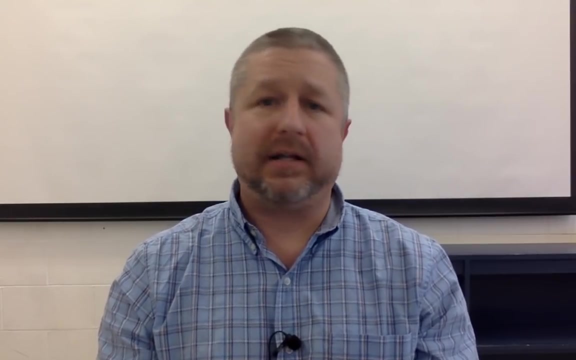 up there, when I record this, when I put this online later- But I don't know what I'm saying, This is online already- I'll go back and put a link up there. I'm going to make a video later this week about five websites and apps that you can use to learn English using the internet. I myself am an 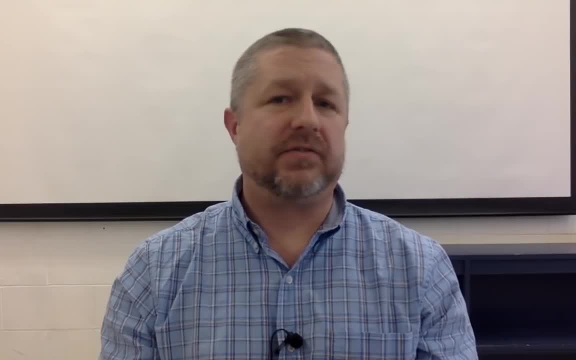 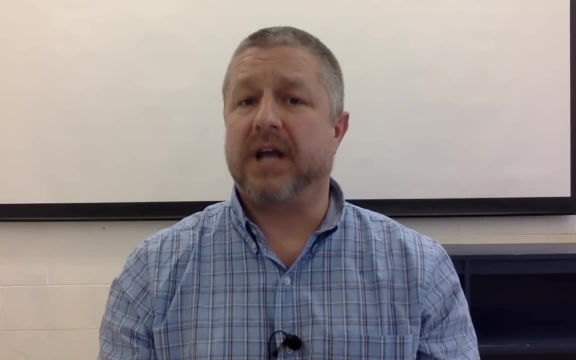 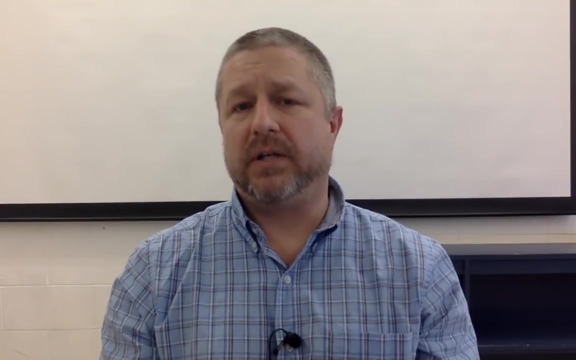 English speaker, but I also speak French. In order to practice French, I'm going to have to go to a French school. I don't have any native speakers near me, So when I practice French, I do it via Skype, And I think Skype is wonderful. If you wanted to immerse yourself in English, if you wanted to surround 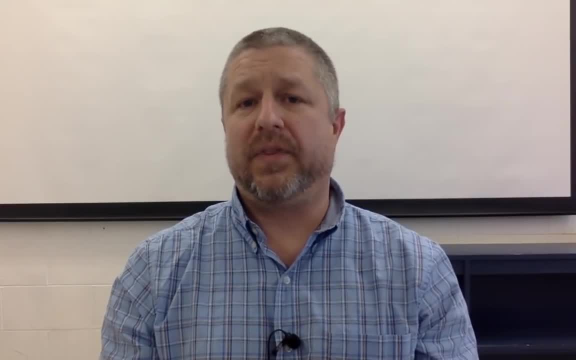 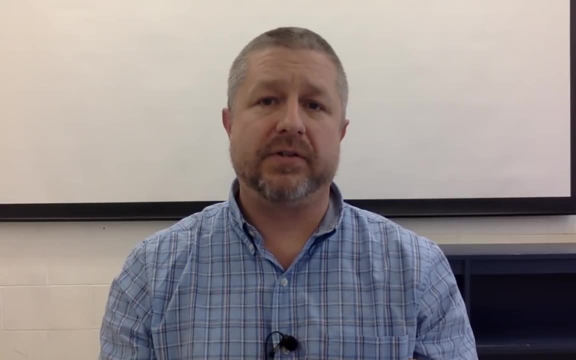 yourself in English. you can certainly do a lot with the internet. You can find books to read in English. You can find YouTube channels like this YouTube channel and many others to listen to English. You can use Skype to have a two-way conversation. 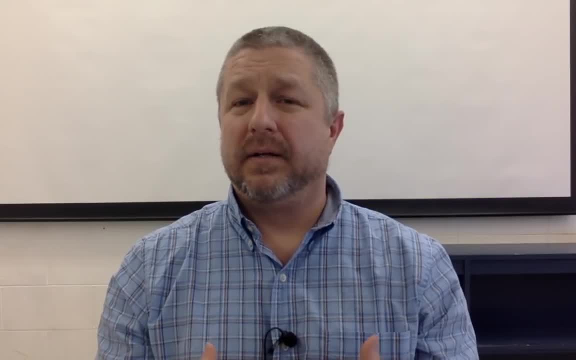 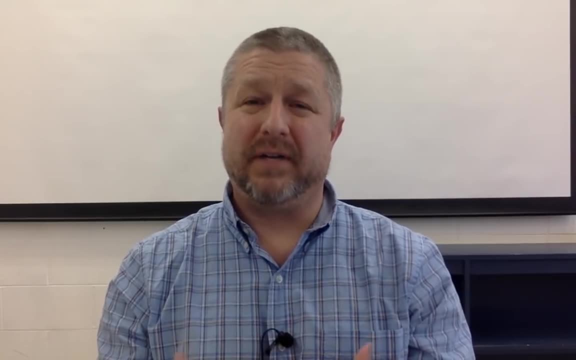 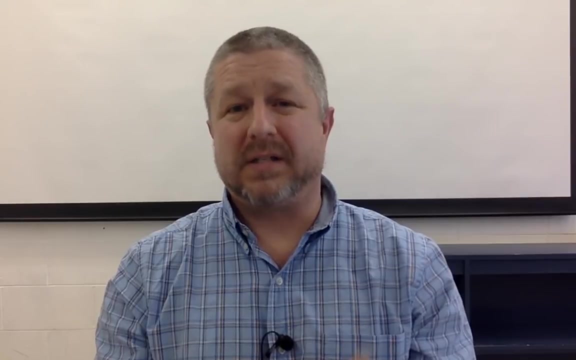 It certainly is a great place. Building a solid base using the internet works well, And you should probably at some point move or live in another country for at minimum a year. So great question: You can do a lot just with the internet, but going abroad does help quite a bit. 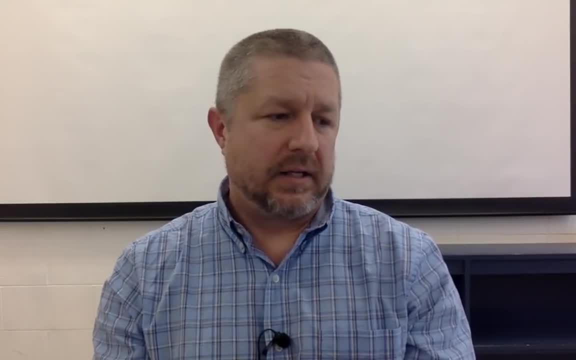 Yeah, and the follow-up question from Rez is: can I be fluent without traveling at all? I think you can. I think 10 or 20% of the time you can. I think 10 or 20% of the time you can. I think 10 or. 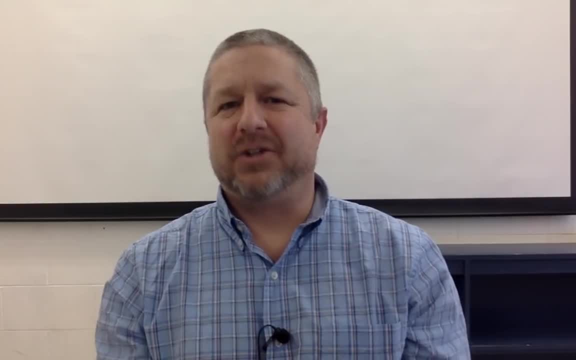 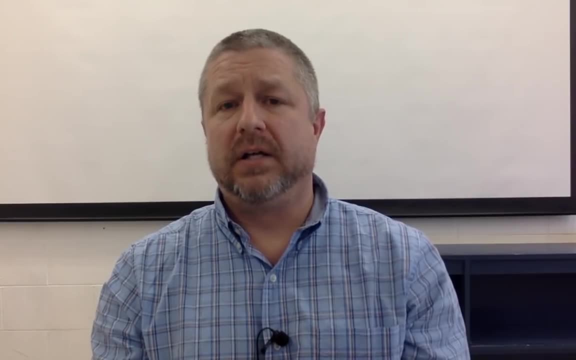 20 years ago. you see how I got to use time there. 10 or 20 years ago I think it would have been a challenge, But I think right now you can do a lot with the internet. You can learn so much and for 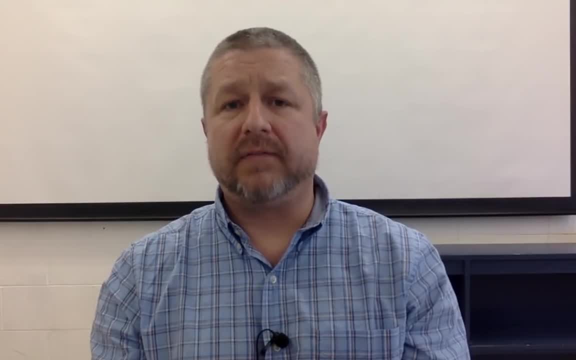 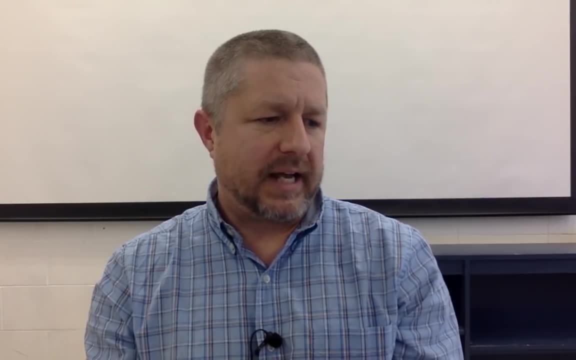 relatively cheaply or for very little money, if not free. What is the difference? This is from Zyvex. What is the difference between must and have to? Well, okay, let me give two sentences, two examples of that. So I must eat. 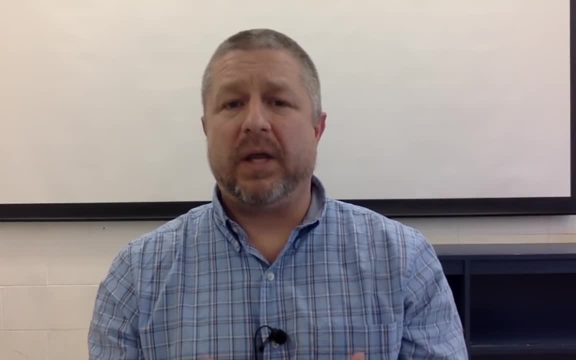 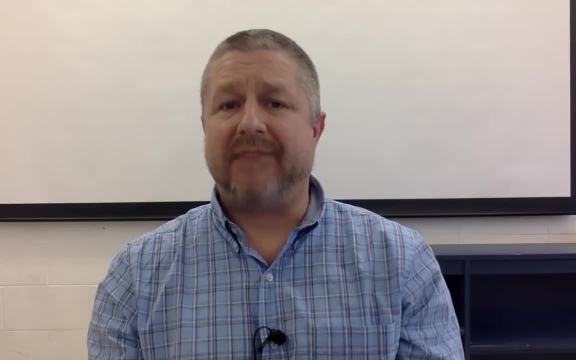 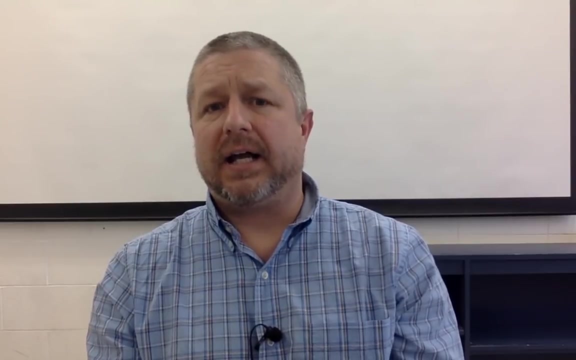 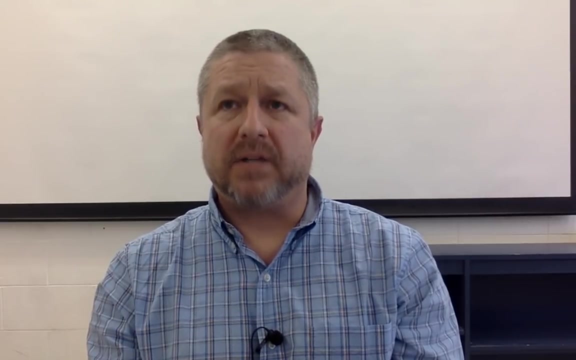 every day. I have to eat every day. Those two sentences mean exactly the same thing. I must go to work, I have to go to work. Those two sentences mean exactly the same thing Just off the top of my head. I can't think of an example where they mean something different. I must get groceries. I have 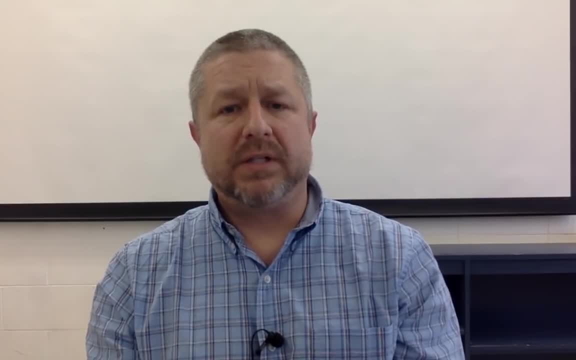 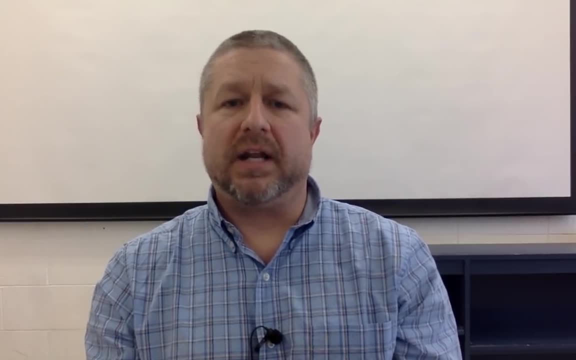 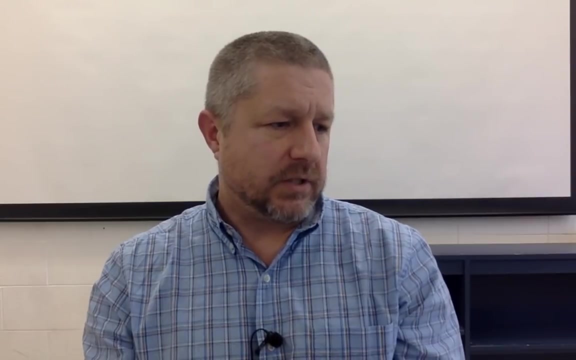 to get groceries. You know I must get groceries. May seem a little more urgent. You know I must eat to live. Might be a little more urgent than I have to eat to live. So very similar though You can use both interchangeably. So I'm just looking over. 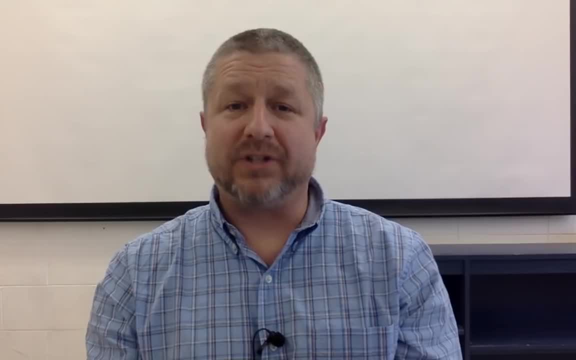 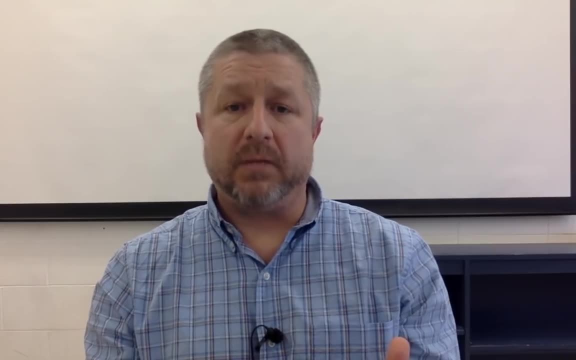 here. I don't have any more questions in the chat. I was planning for this live stream to be about 15 minutes long and it's almost 20.. If there are any more questions, please ask them, And don't forget to look towards the end of this week. I will be putting together a video for you. I'm going to be 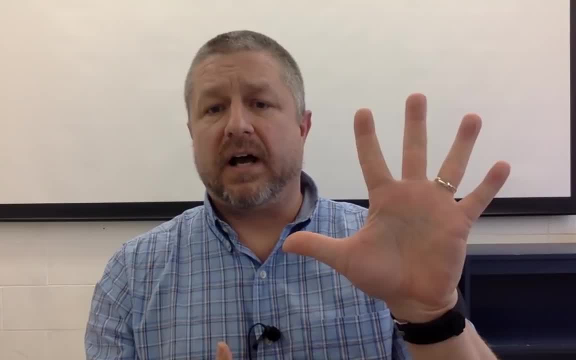 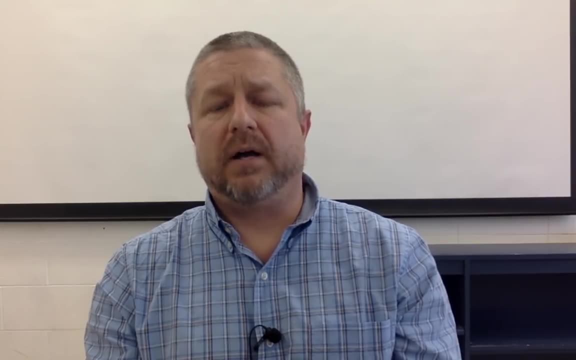 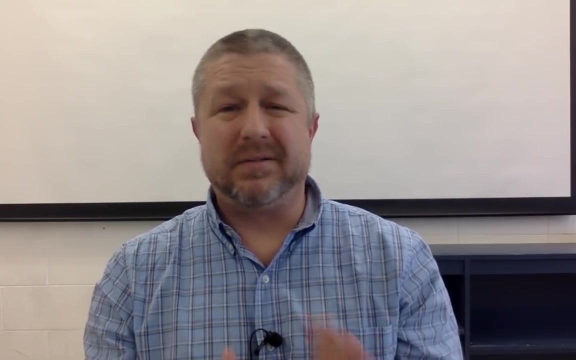 posting a video about five apps and websites that you can use for free. They're all free. That can really help you with your English. I'll make sure I get that up towards noon Eastern Standard Time on Saturday somewhere in there, but with some flexibility It might be later in the day than 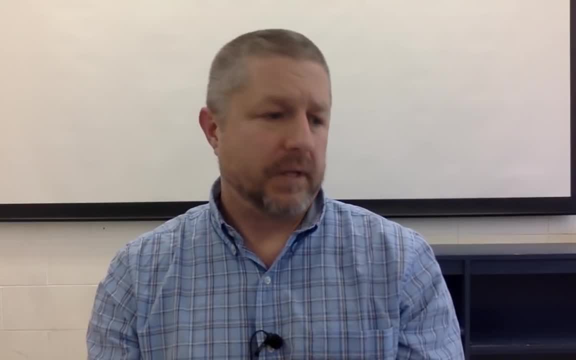 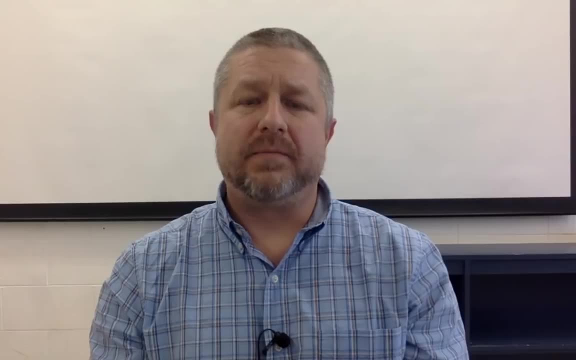 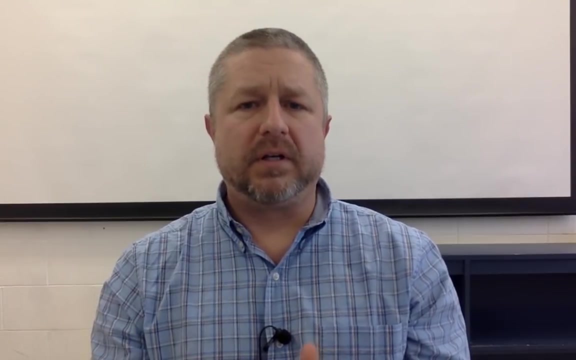 that, But I'm planning to shoot that video later this week. Yeah, no problem, There's a thanks in the chat. It's no problem. Planning to do another live stream next week, Tuesday at 4 pm Eastern Standard Time. I'm going to. 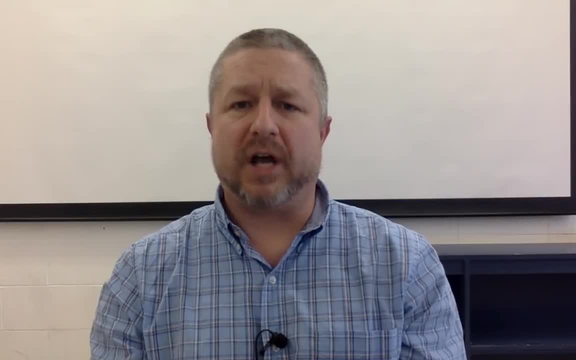 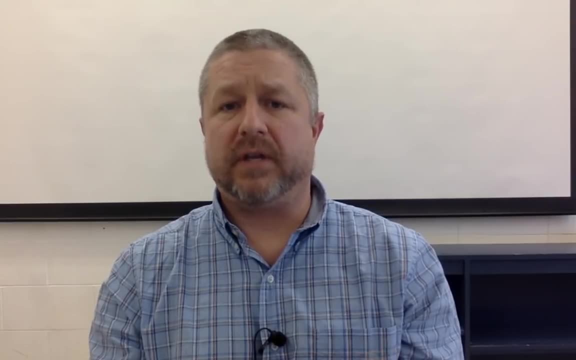 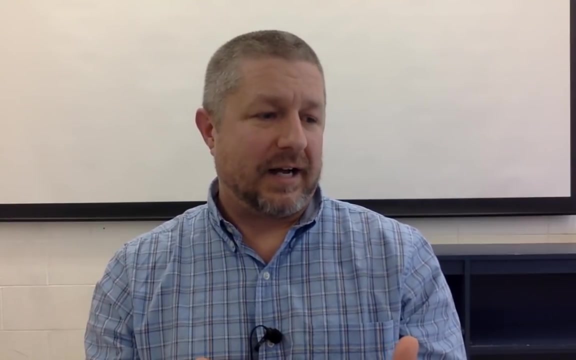 kind of look at the time zones to see when is a good time to do live streams, So I might play around with when it happens. But certainly once the live stream is over, the video is available to all of you that come later. So anyways, thank you very much. It was great. I got up to four viewers. 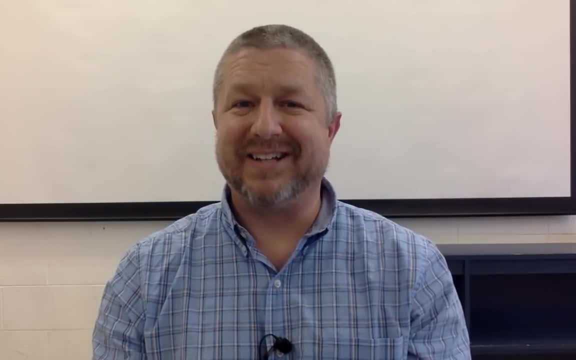 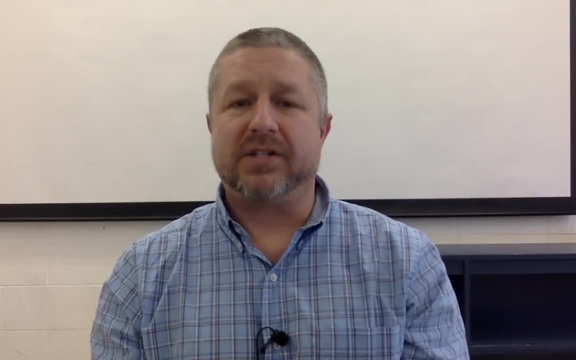 which for me is amazing. I know you might might not sound like a lot, but for me that just made me super happy to see people watching And to all those people who are watching later, it's just so cool for me to look at all the different 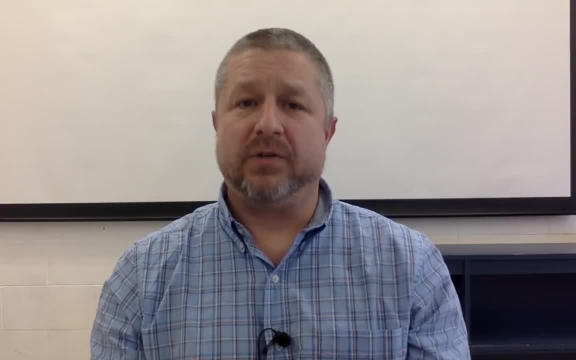 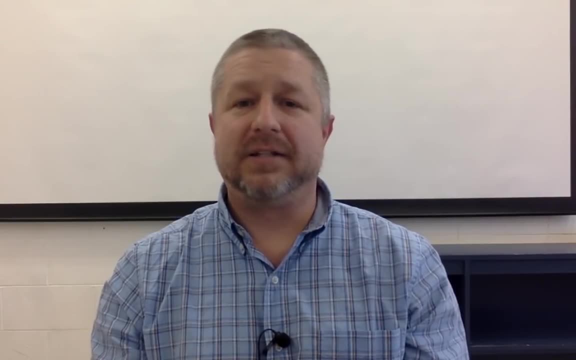 countries in the world that visit and watch my YouTube videos. So if you're out there in India, if you're out there in China, if you're out there in Algeria, if you're out there in Spain, Japan, Korea- I can't list them all, But thank you so much for watching. Let me just check if there's any.